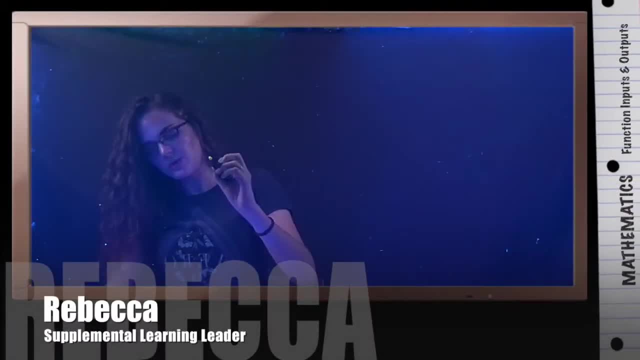 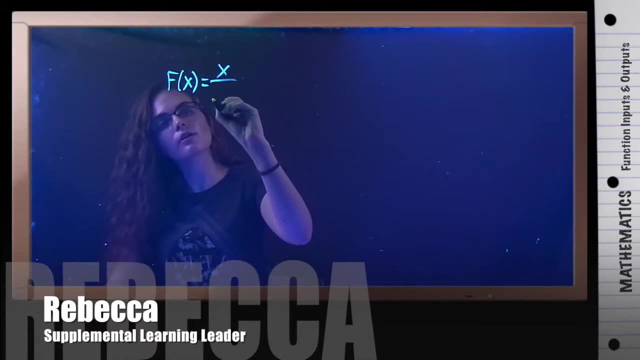 For this example, we're going to evaluate f of x equals x over x minus 2.. We're going to evaluate f of 0,, f of 1, f of 2, and we need to find x when f of x equals 5.. So first, 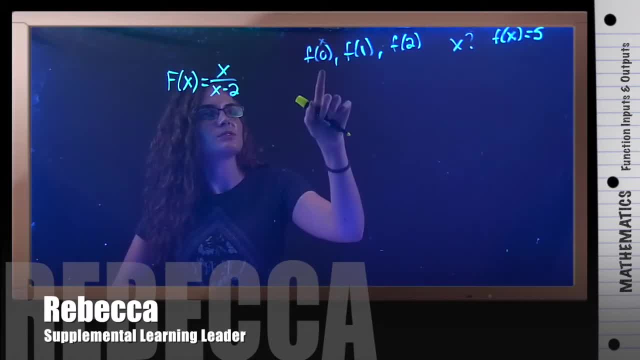 when we find f of 0, we know that x must be 0 because it's inside. So this is the same thing as saying x equals 0.. So we're going to plug in x for 0 here and we get 0 over 0 minus 2.. And any time you have 0 on the top of a fraction, you know. 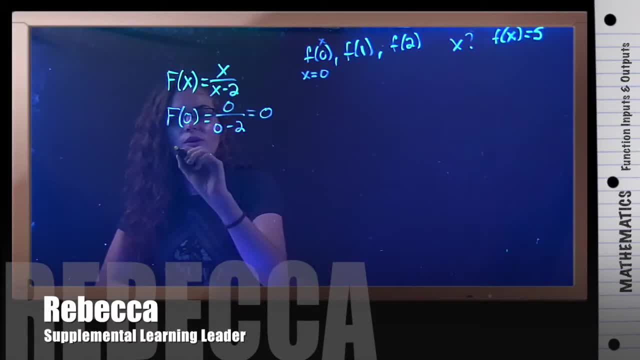 your answer is just going to be 0.. So we know f of 0 equals 0.. So that's our first answer. Now our second one is going to be f of x equals x over x minus 2.. So we're going to. 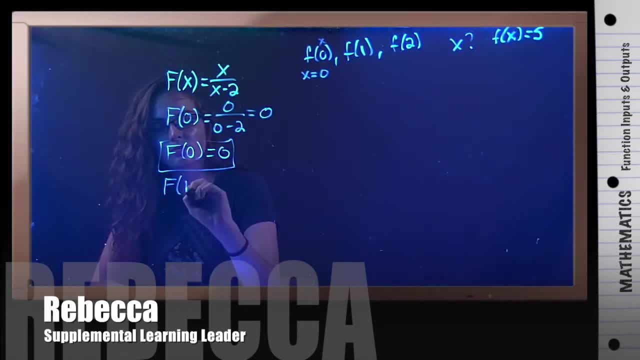 find f of 1. So we can plug in 1, because x equals 1. So we can plug in 1 wherever we see x, 1 over 1 minus 2.. Here we get 1 over negative 1. And 1 divided by negative 1 is: 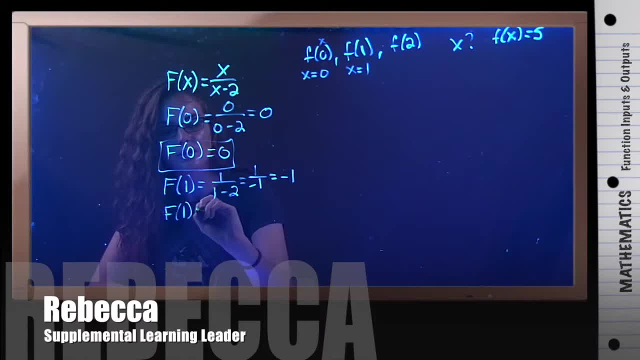 negative 1. So f of 1 is negative 1.. So that's our second answer. Now we have to find f of 2.. f of 2, we plug in 2 wherever we see x, So 2 over 2 minus 2.. Now we get 2 over 0. But 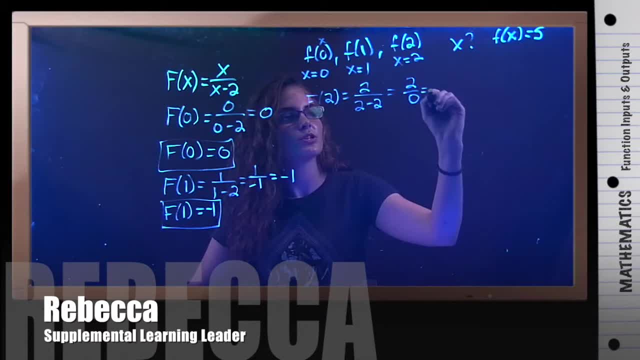 any time you have 0 on the denominator of a fraction, your answer is undefined. So that's our third answer. Now we have to find x when f of x equals 5.. So this is saying something different. This doesn't tell us that x is 5.. It tells us that f of x is 5.. So, instead of plugging,